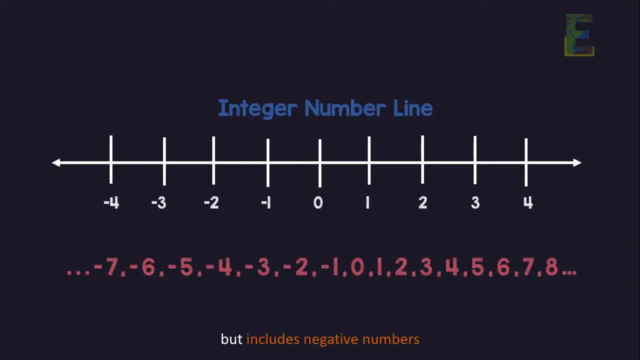 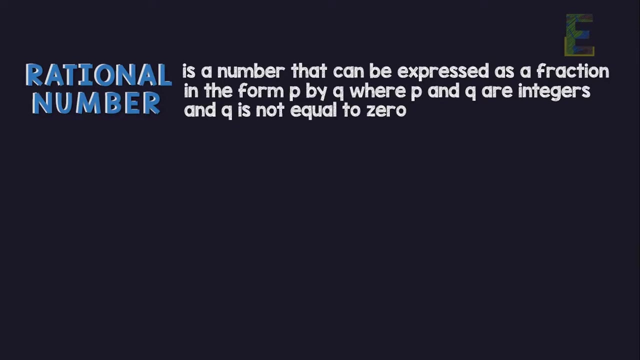 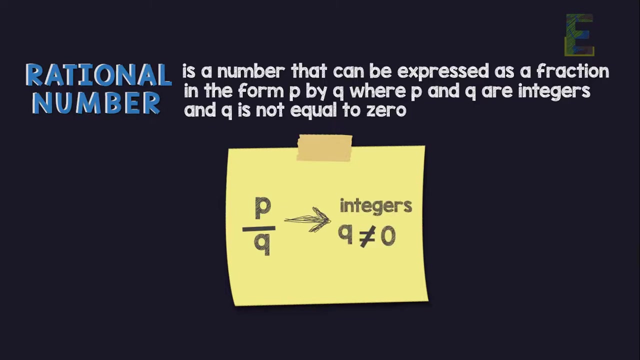 integer is that integer is like a whole number but includes negative numbers. So that's the quick review of integers. Now let's discuss what rational number is. Rational number is a number that can be expressed as a fraction in the form p by q, where p and q are integers and q is not equal to zero. 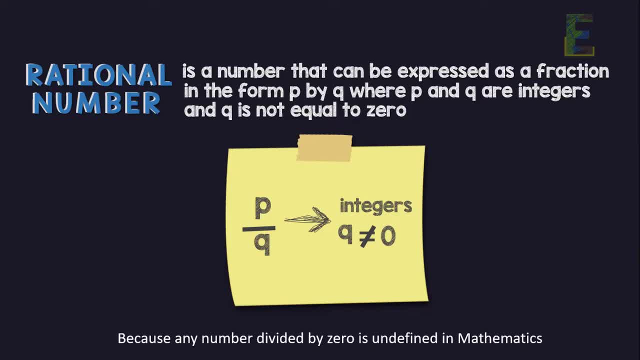 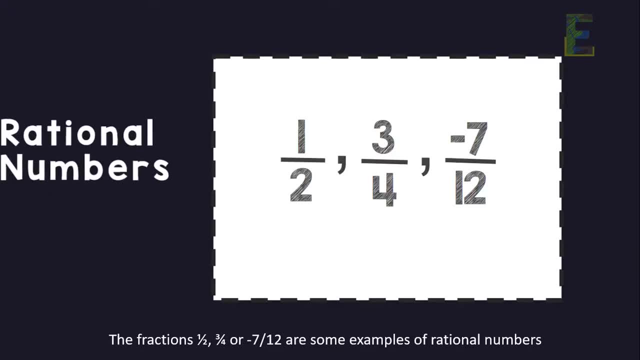 because any number divided by zero is undefined in mathematics. So the fractions one, half, three, fourth or negative seven over twelve are some examples of rational numbers. The numbers notice that the numerator and denominator are integers and the denominator is not equal to 0. now the question is: is an integer a rational? 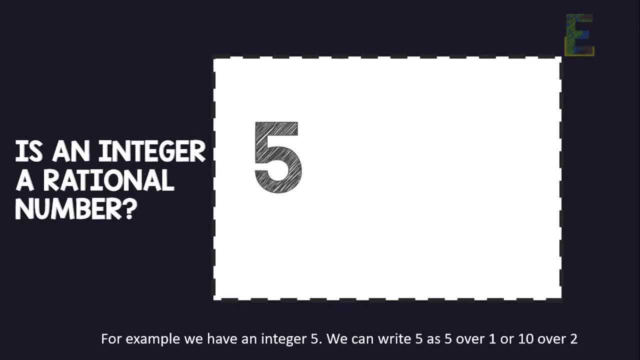 number. for example, we have an integer 5. we can write 5 as 5 over 1 or 10 over 2. it can be written as fraction. therefore, 5 is a rational number. now how about the integer negative 8? is it a rational number? negative 8 can be written as: 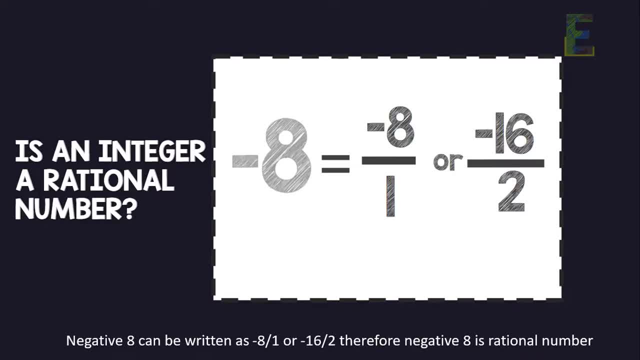 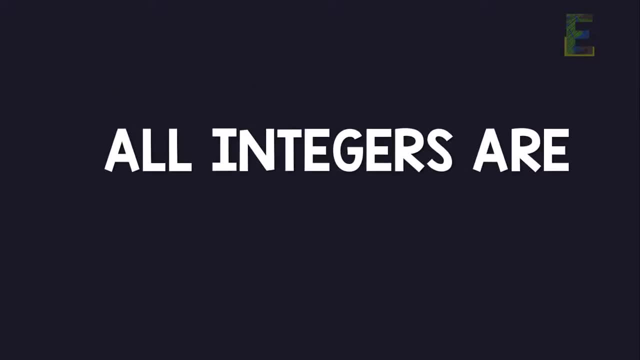 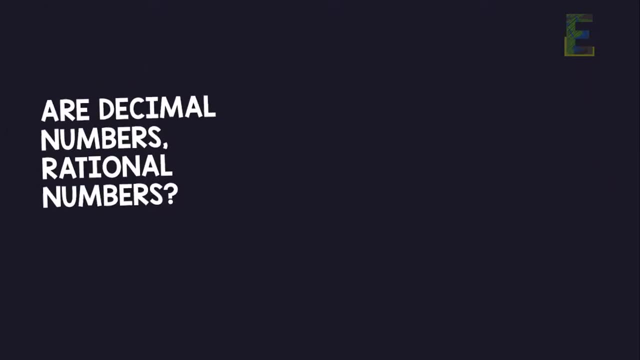 negative 8 over 1 or negative 16 over 2. therefore, negative 8 is a rational number. based on the examples, we can conclude that all integers are rational numbers. now how about decimal numbers? are decimal numbers rational numbers? for example, we have a decimal 0.50. we. 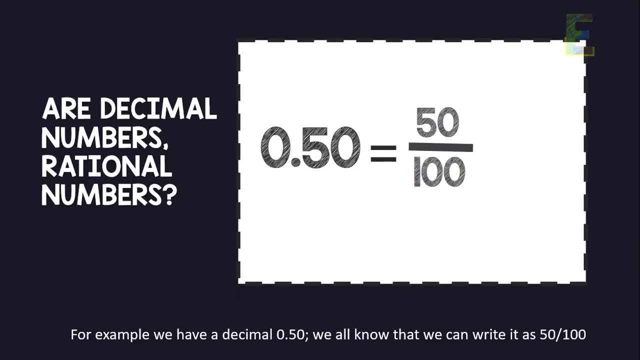 also have a decimal 0.50, and we can be any decimal for any decimal. we can also know that we can write it as 50 over 100 or one half in simplified form. therefore it is also a rational number. now another example: what if we have a repeated decimal like 0.3333 and so on? 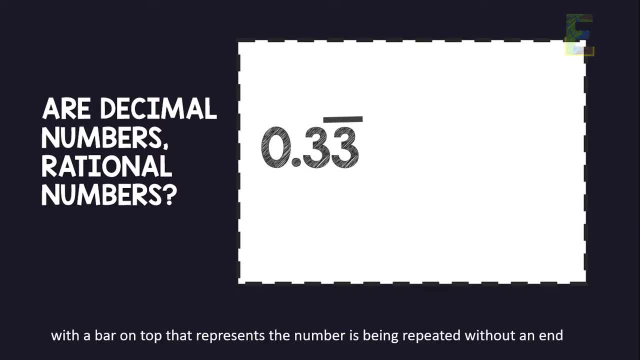 or we can write it as 0.33 with a bar on top that represents the number is being repeated without an end. is this also a rational number? so the decimal number 0.333 and so on is one-third if written in fraction. therefore, repeating decimals are also rational numbers. so far all the examples we have. 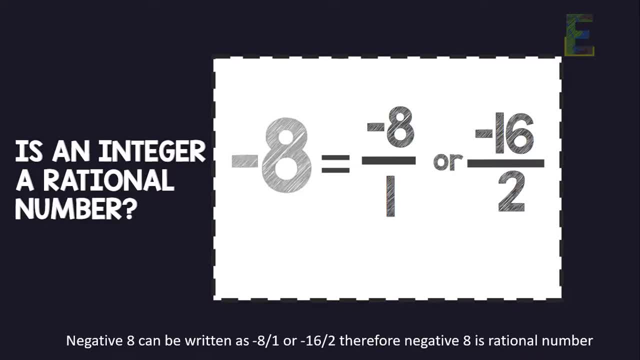 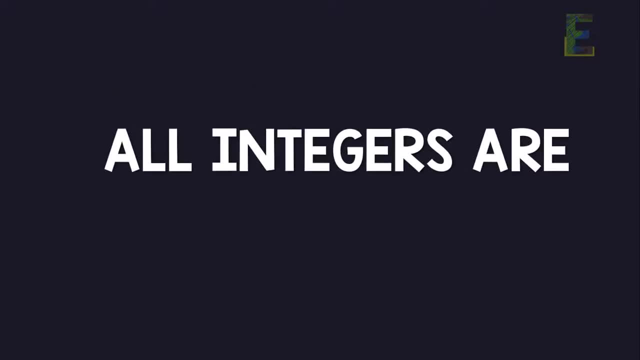 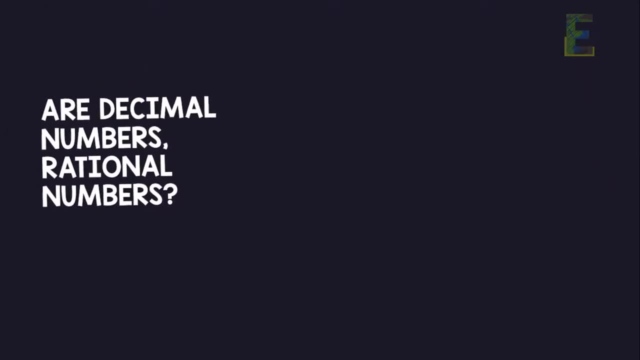 as negative 8 over 1 or negative 16 over 2.. Therefore, negative 8 is a rational number. Based on the examples, we can conclude that all integers are rational numbers. Now how about decimal numbers? Are decimal numbers rational numbers? For example, we have a decimal 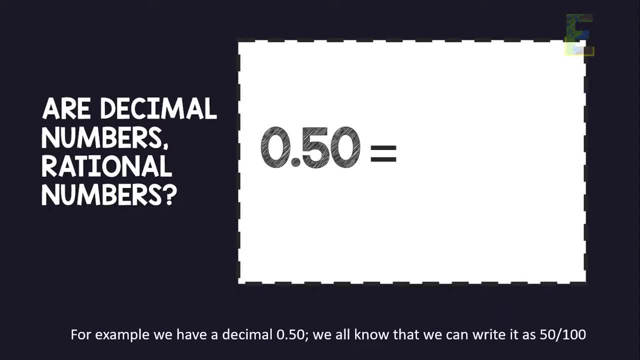 zero, 0.50.. We all know that we can write it as 50 over 100 or one half in simplified form. Therefore it is also a rational number. Now another example: what if we have a repeated decimal like 0.33333 and so on? or we can write it as 0.33 with a bar on top that represents the. 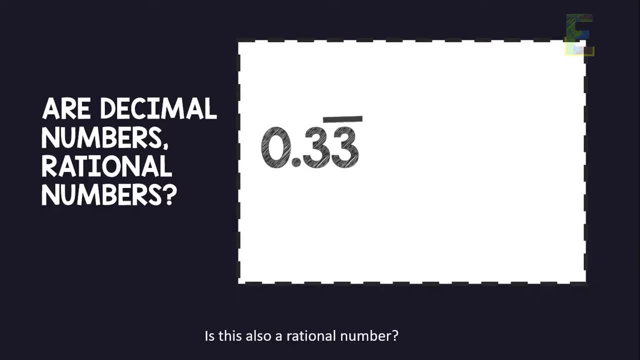 number is being repeated without an end. Is this also a rational number? So the decimal number 0.33333 is a rational number. Now, how about decimal numbers? Are decimal numbers rational numbers? Is this also a rational number? So the decimal number 0.33333 and so on is one third if written. 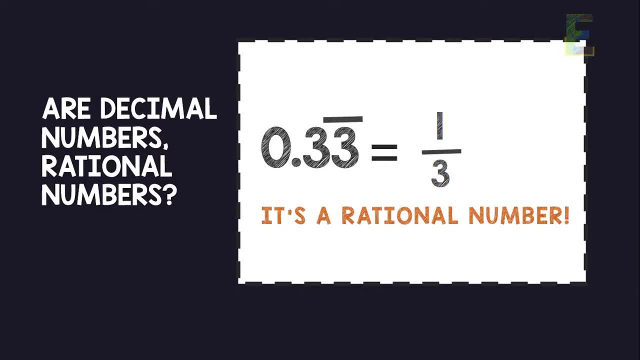 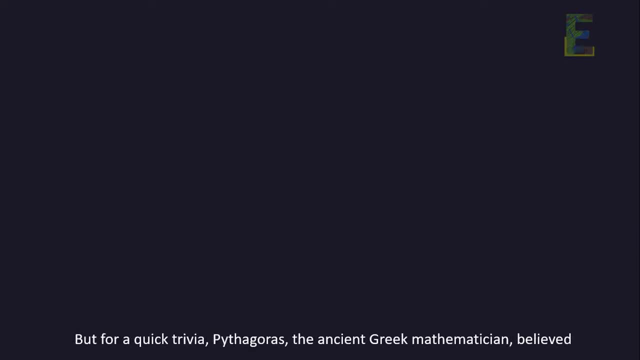 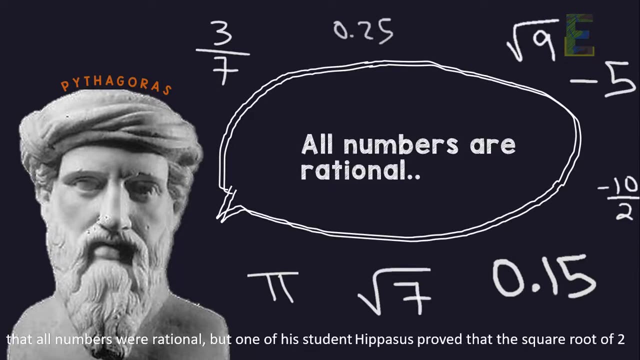 in fraction. Therefore repeating decimals are also rational numbers. So far all the examples we have are rational numbers. But for a quick trivia, Pythagoras, the ancient Greek mathematician, believed that all numbers were rational, But one of his students, Hephasus, 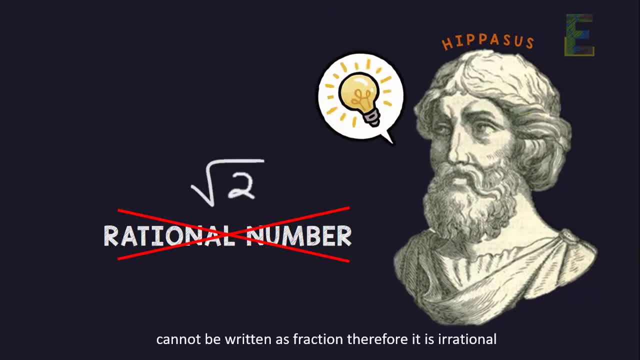 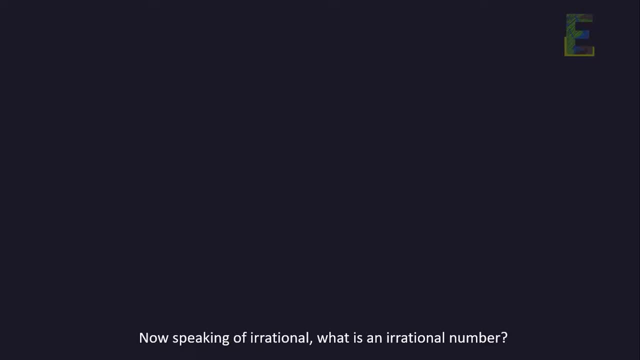 proved that the square root of 2 cannot be written as fraction. therefore, it is irrational. Now speaking of the irrational, what is an irrational number? Irrational number is a real number that cannot be written as a simple fraction like the square root of 2.. If we use 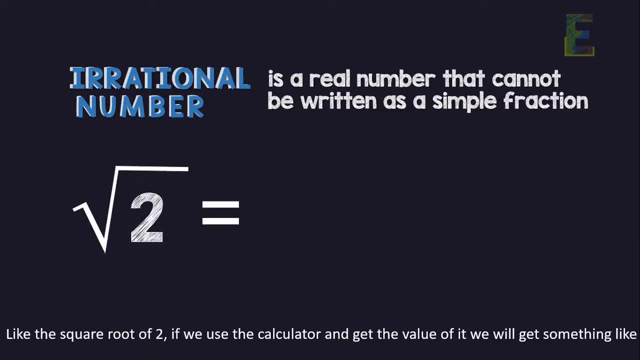 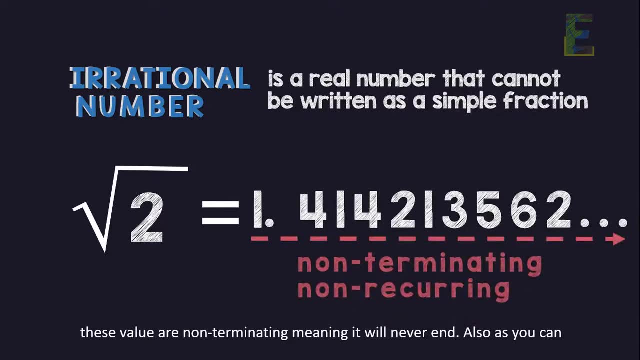 the calculator and get the value of it, we will get something like 1.414213562 and so on. These values are non-terminating, meaning it will never end. Also, as you can see, that the digit in the decimals doesn't have pattern, therefore, this is a non-recurring decimal. This kind of number. 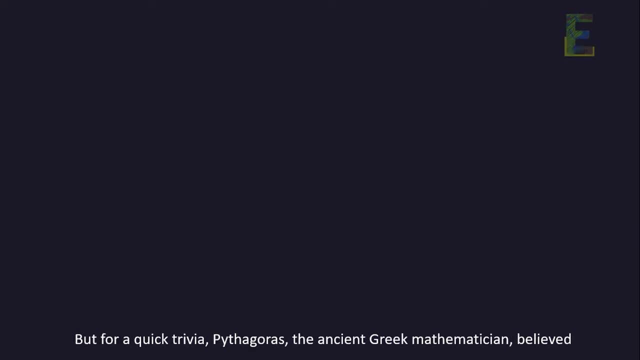 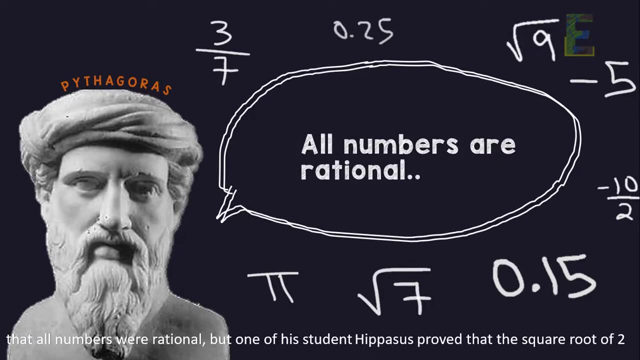 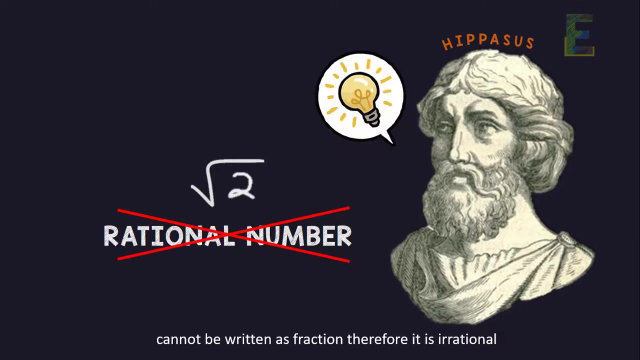 are rational numbers. but for a quick trivia, patagoras, the ancient greek mathematician, believed that all numbers were rational, but one of his student, hepasus, proved that the square root of 2 cannot be written as a fraction. therefore it is irrational. now, speaking of the 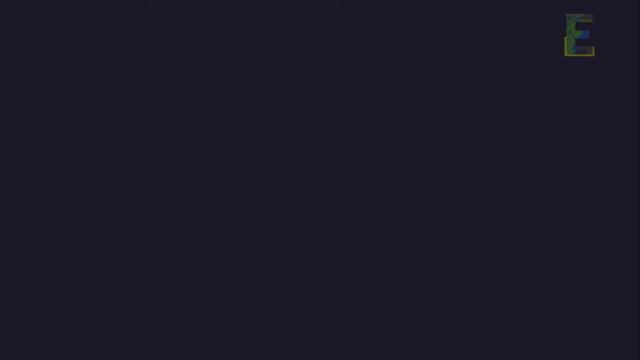 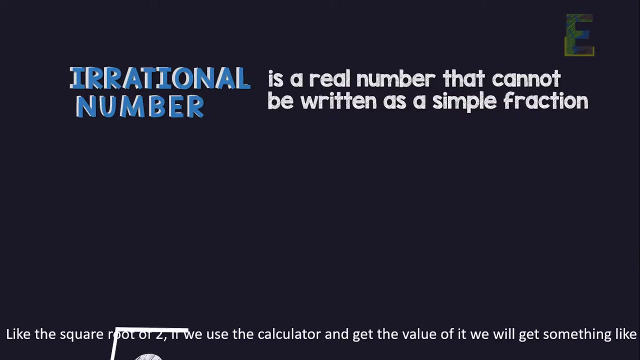 irrational. what is an irrational number? a rational number is a real number that can't be written as a simple fraction like the square root of 2. if we use the calculator and get the value of it, we will get something like one point four, one, four, two, one three, five, six, two and so on. this value of 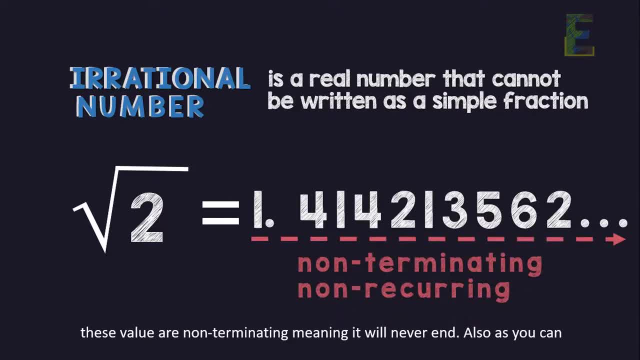 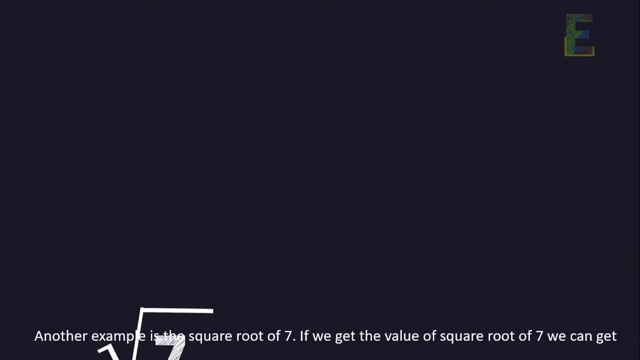 are non-terminating, meaning it will never end. also, as you can see, that the digit in the decimals doesn't have pattern. therefore this is a non-recurring decimal. this kind of number is called irrational number. another example is the square root of 7. if we get the value of square root of 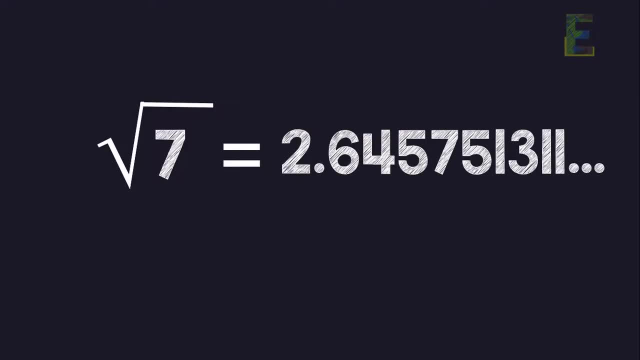 7, we can get something like 2.645751311 and so on. this is also a non-terminating and non-recurring decimal number and we cannot write it into fraction. therefore, it is also an example of irrational number, but we cannot say that all square root numbers are irrational, because 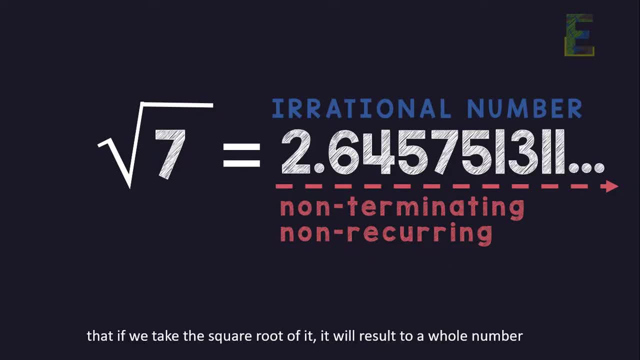 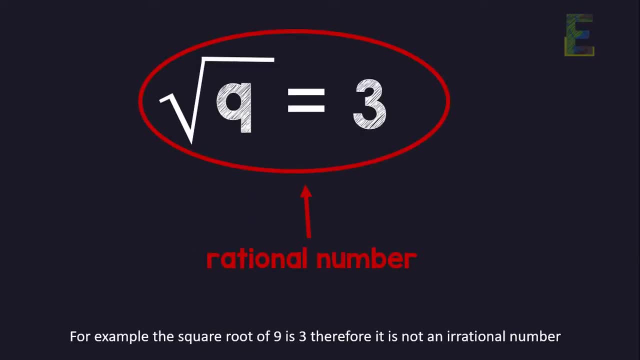 there are some numbers that if we take the square root of it, it will result to a whole number. for example, the square root of 9 is 3. therefore it is not an irrational number. in fact, square root of any perfect square number will be rational numbers. 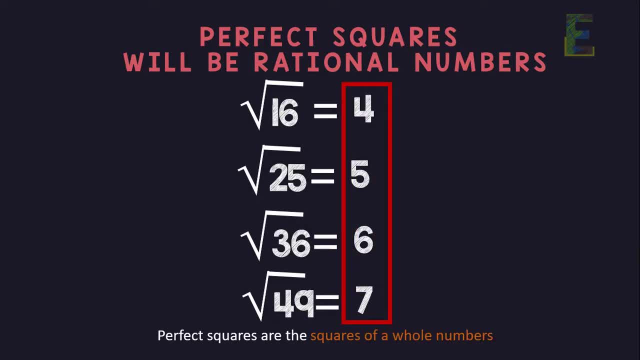 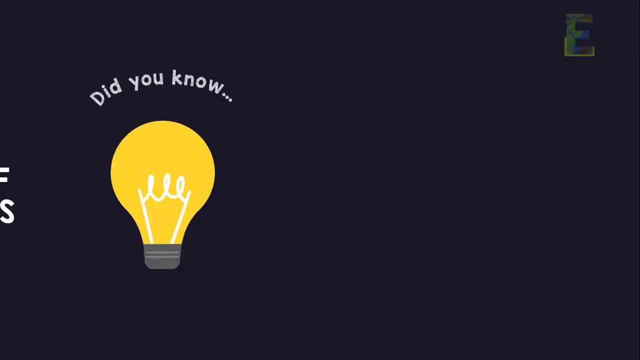 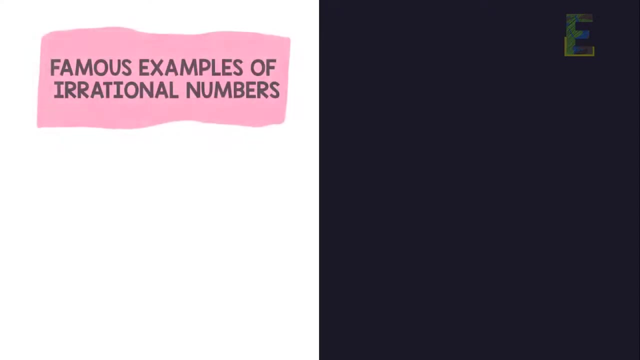 perfect squares are the squares of a whole number. and did you know that there are some famous examples of irrational numbers? yes, you've heard it right, and here are some famous examples of irrational numbers. first is the pi. many mathematicians calculated the value of pi over quadrillion decimal places. but 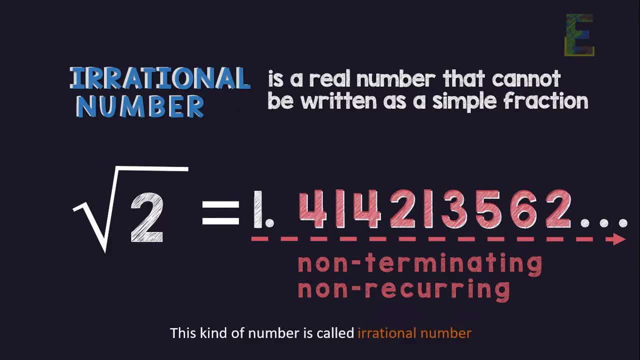 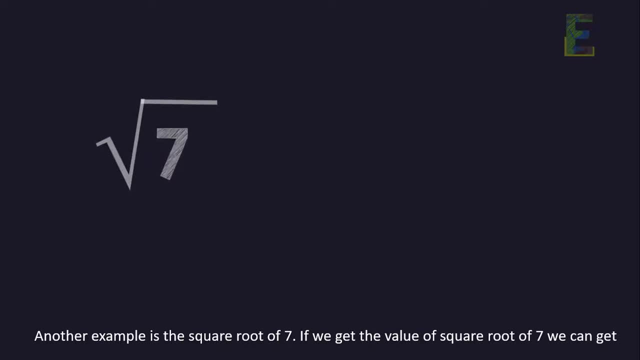 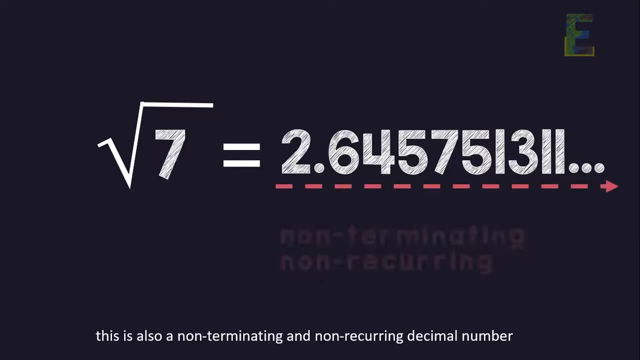 is called irrational number. Another example is the square root of 7.. If we get the value of square root of 7, we can get something like 2.645751311 and so on. This is also a non-terminating and non-recurring decimal number And we cannot write it into fraction. therefore, it is also. 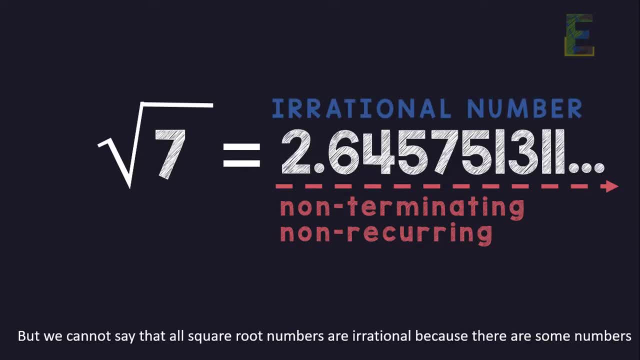 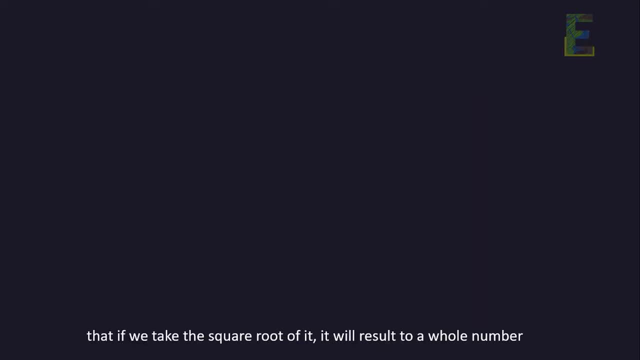 an example of irrational number. But we cannot say that all square root numbers are irrational, because there are some numbers that if we take the square root of it it will result to a whole number. For example, the square root of 9 is 3, therefore it is not an irrational number. In fact, 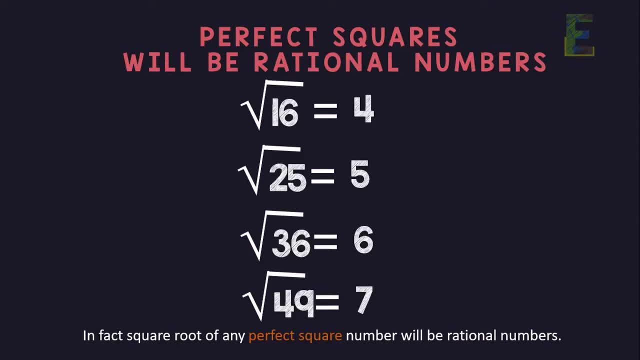 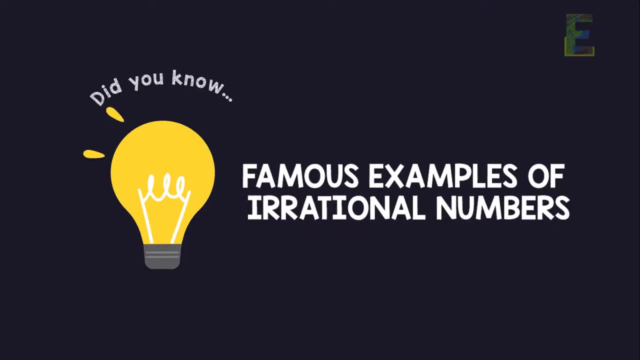 square root of any perfect square number will be rational numbers. Perfect squares are the squares of a whole number. And did you know that there are some famous examples of irrational numbers? Yes, you've heard it right, And here are some famous examples of irrational numbers. First is the pi. Many mathematicians. 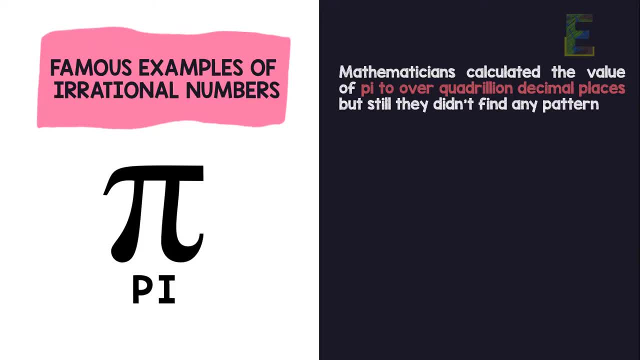 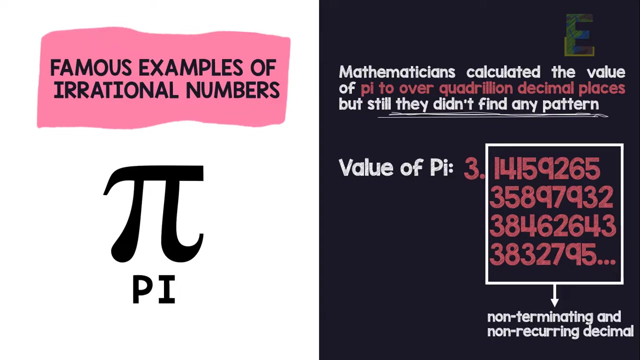 calculated the value of pi to over quadrillion decimal places, but still they didn't find any pattern. The value of pi is 3.14159265358979323846264338.. Therefore, it is a non-terminating, non-recurring decimal and it is an example of irrational. 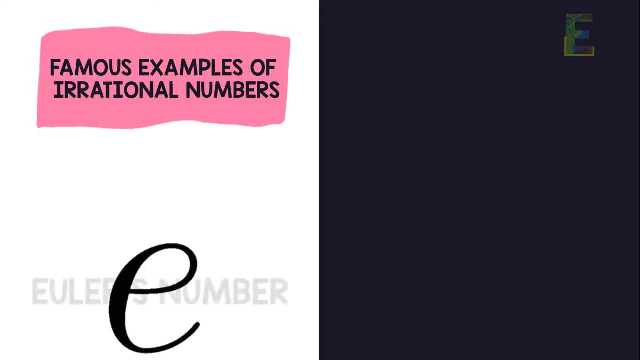 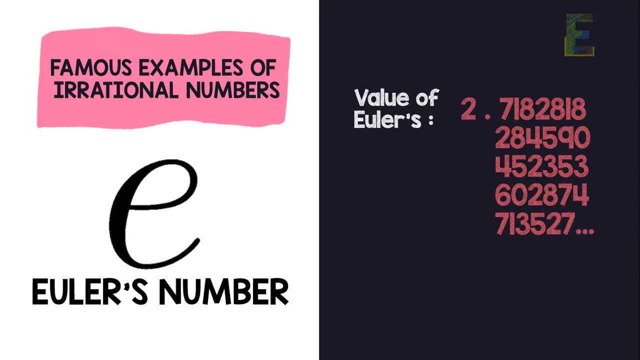 number. Next is the Euler's number. The value of Euler's number is 2.7182818284590452353602874713527 and so on, And many mathematicians also have calculated Euler's number to lots of decimal places, but still no pattern is showing. Therefore it is an irrational number. 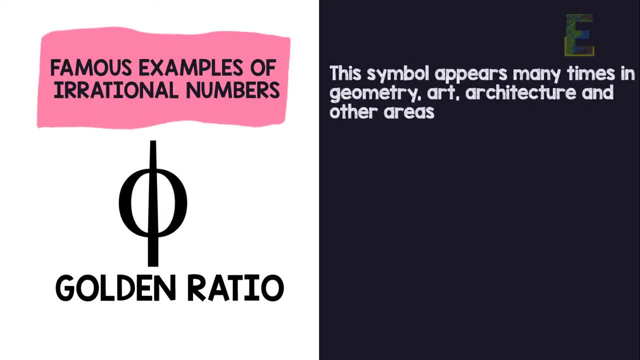 Next famous example is the golden ratio. Golden ratio appears many times in geometry, art, architecture and other areas, And it is a special number which has a value of 1.61803398874989484820 and so on, and still no pattern and no ending. 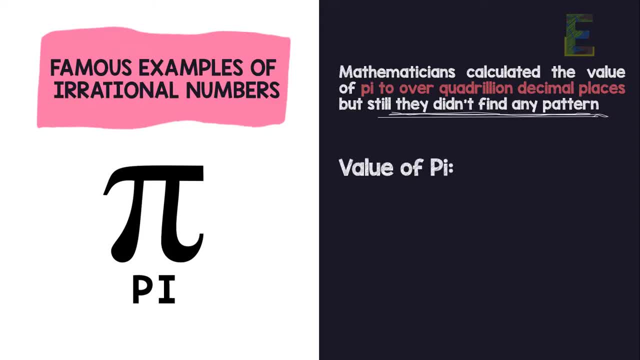 still they didn't find any pattern. the value of pi is 3.1415926535897932384626433832795, and so on. therefore, it is a non-terminating, non-recurring decimal and it is an example of irrational number. next is the Euler's number. the value Euler's number is two point seven, one, eight, two, eight one. 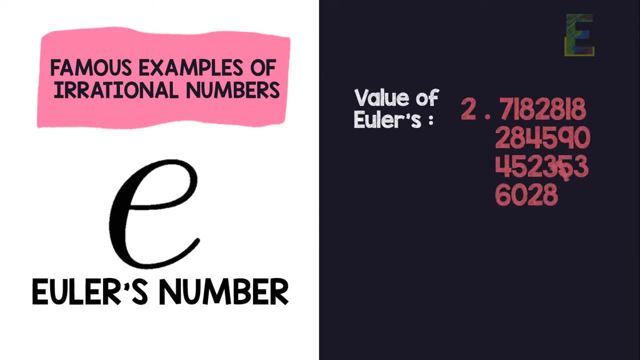 eight, two, eight, four, five, nine, zero, four, five, two, three, five, three, six, zero, two, eight, seven, four, seven, one, three, five, two, seven and so on. and many mathematicians also have calculated Euler's number to lots of decimal places, but still no pattern is showing. therefore it is an irrational number. 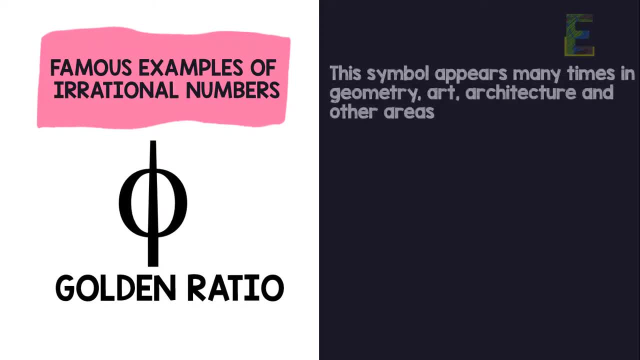 next famous example is the golden ratio. golden ratio appears many times in geometry, art, architecture and other areas, and it is a special number which has a value of one point: six, one, eight, zero, three, three, nine, eight, eight, seven, four, nine, eight, nine, four, eight, four, eight, two, zero and so. 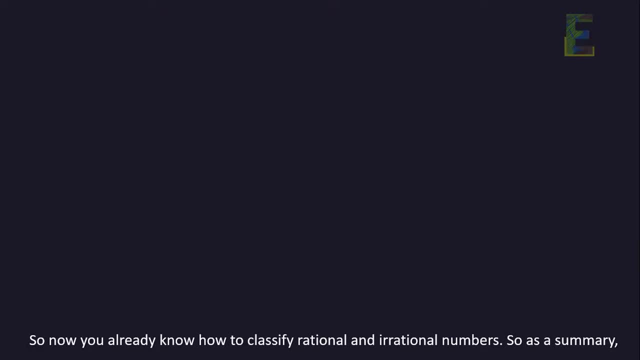 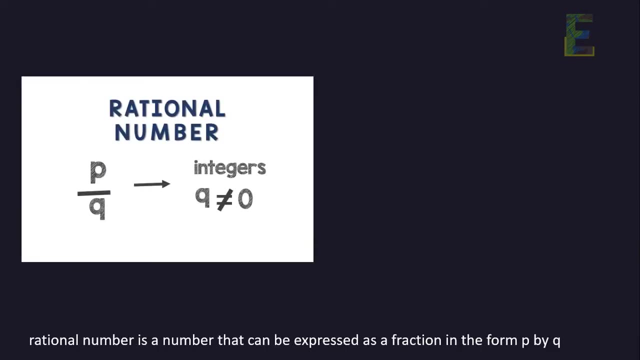 on and still no pattern and no ending. so now you already know how to classify rational numbers and irrational numbers. so, as a summary, rational number is a number that can be expressed as a fraction in the form P by Q, where P and Q are in integers and Q is not equal to zero. and irrational number is a real number that cannot be written as. 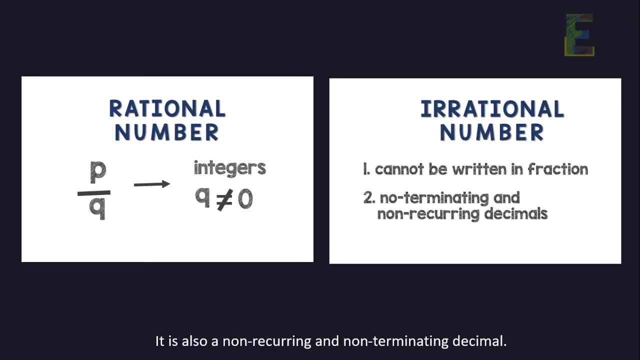 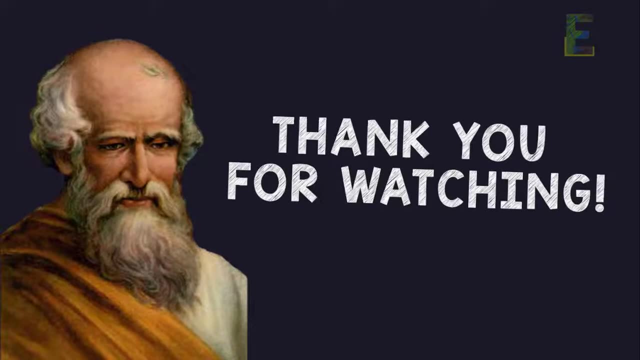 a simple fraction. it is also a non-recurring and non-terminating decimal. famous examples are pi, Euler's number and golden ratio. also, the square root of a non-perfect square. numbers are example of irrational numbers. so that's it, guys. did you enjoy our topic for today? I hope you learned a. 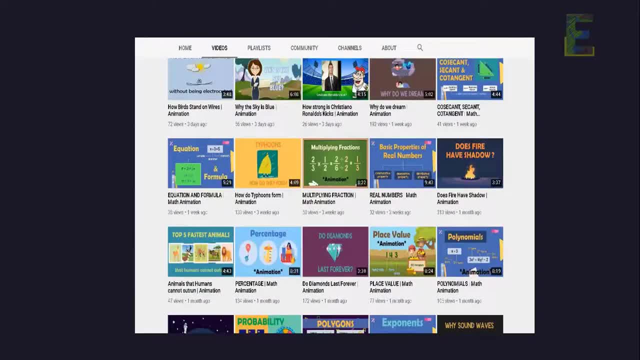 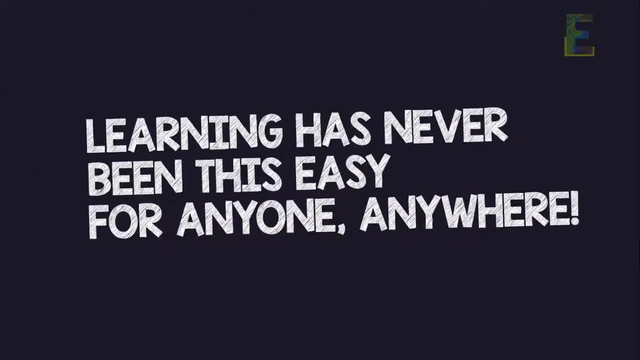 lot about rational and irrational numbers also. you can watch our other video tutorials here in our channel. once again, this is earth. pen learning has never been this easy for anyone anywhere. have a nice day.